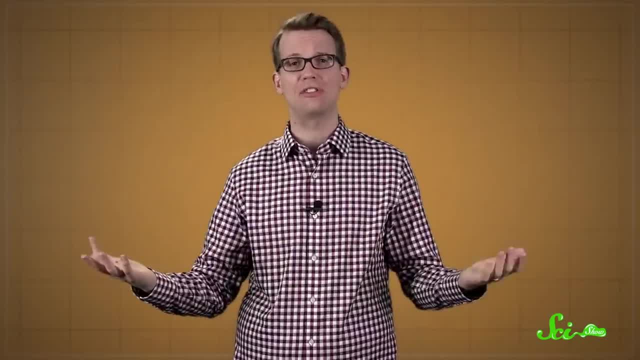 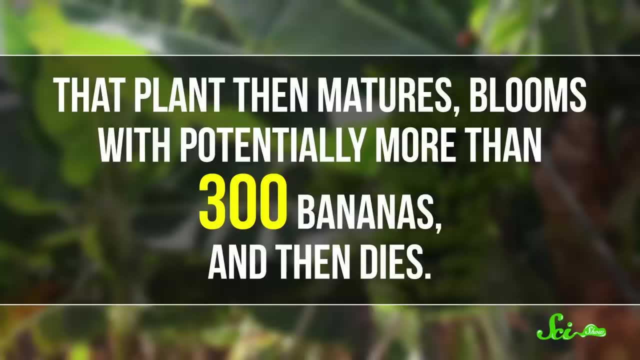 good, taste good and be easy to grow, So most banana plants live a chaste life. If you're a banana farmer, you get more banana plants by cutting off a piece of the stem of an existing plant and then sticking it in the ground. That plant then matures, blooms with potentially more than 300 bananas and then dies. Because they're all the same, they're super vulnerable to disease. There's no chance that one banana plant will happen to have a gene that makes it resistant. 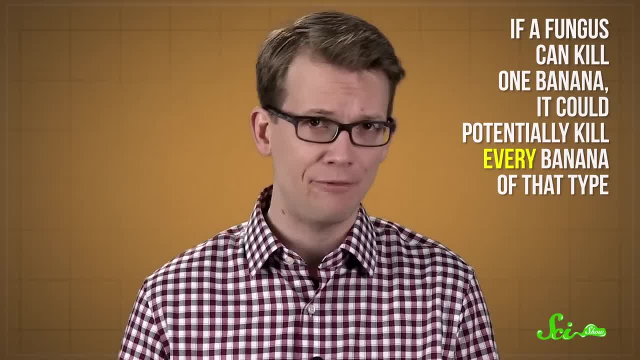 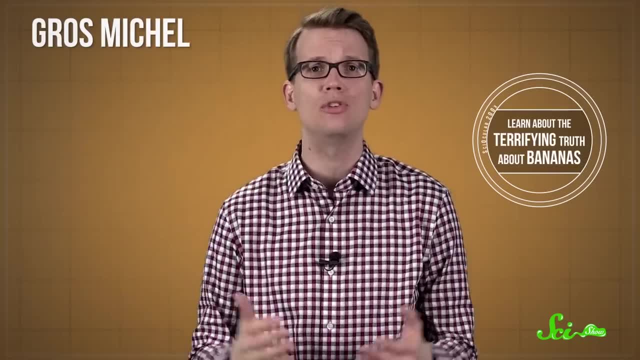 So if a parasite or fungus can kill one banana, it could potentially kill every banana of that type. That's something that's happened before. Back in 2013,, we here at SciShow talked about how the Gros Michel banana, which was bigger, 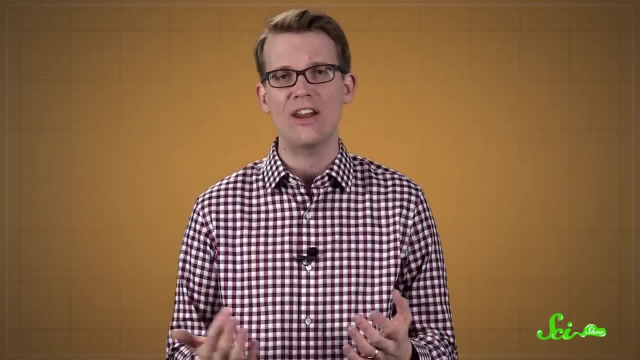 sweeter and hardier than the Cavendish, went virtually extinct in the 1950s. The culprit was a highly infectious fungus we called a panamodium. So if you're a fan of bananas, you know what I'm talking about, If you're a fan of bananas. 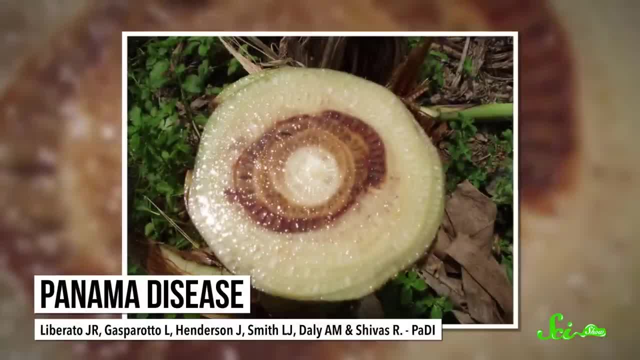 you know what I'm talking about. If you're a fan of bananas, you know what I'm talking about. In the space of about 10 years, Panama disease reduced the Gros Michel from the world's most popular fruit to just another weird thing your grandparents talk about, but nobody else. 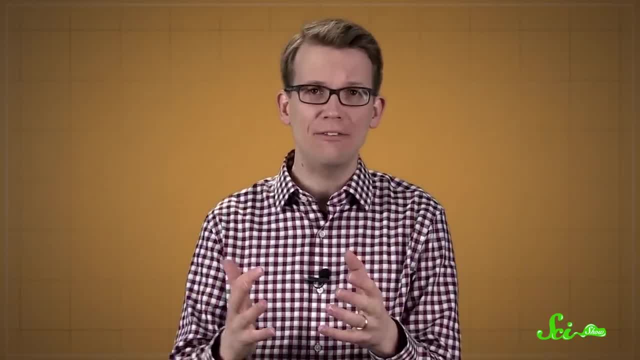 remembers. And the banana industry would have died with the Gros Michel if it weren't for the last minute switch to the Cavendish. While it wasn't as big and it didn't taste the same as the Gros Michel, the Cavendish- 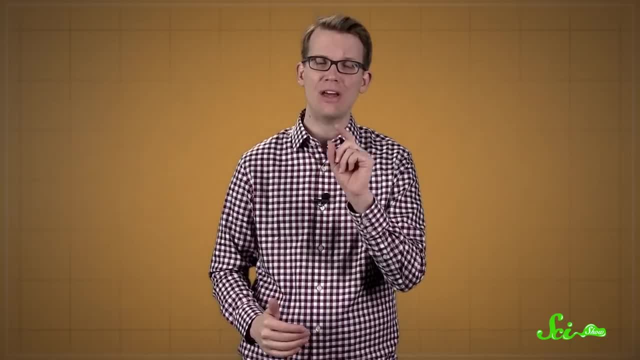 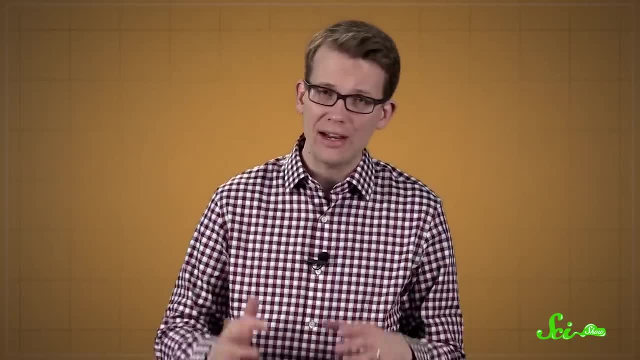 was immune to Panama disease, at least the type of Panama disease that was around at that time In 2013,, we also told you that a new strain of Panama disease had emerged that could infect the Cavendish, but that it would probably be fine. Infected fields were being quarantined. scientists were working on developing. 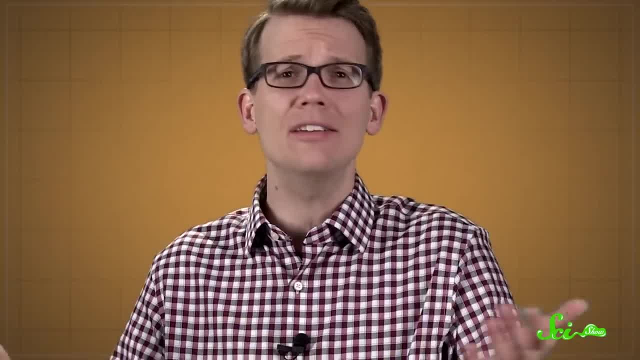 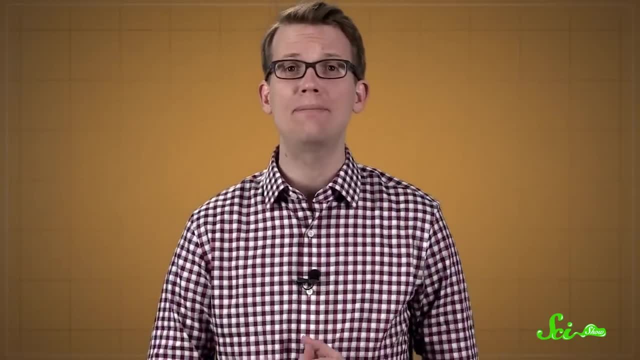 a new kind of Cavendish that could resist the new disease. and hey, we had the lessons of history. We weren't gonna let what happened to the Gros Michel just happen again, right? So here's an update on that story, According to a study published in November in the journal. 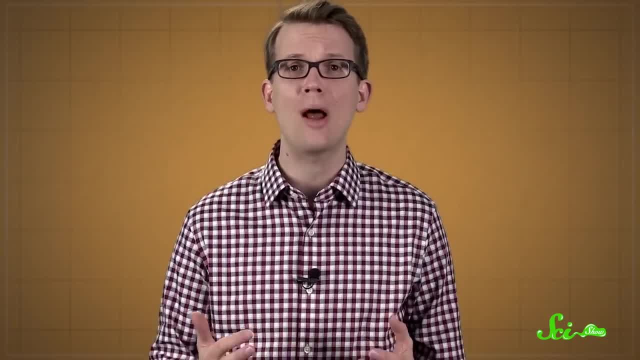 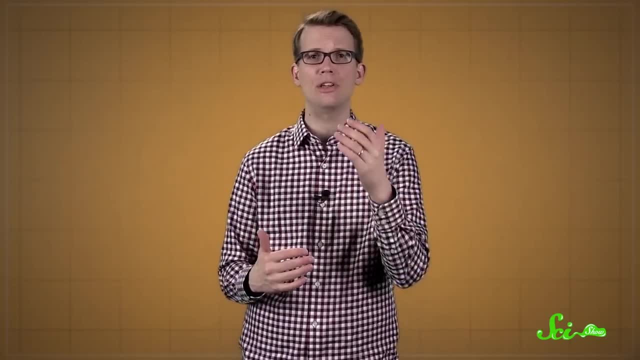 Plus Pathogens, this new strain of Panama disease, known as Tropical Race 4, or just TR4, is spreading. It originated in northern Australia, and the last time we talked about this it was also in Southeast Asia and southern China. Since then, the researchers note that 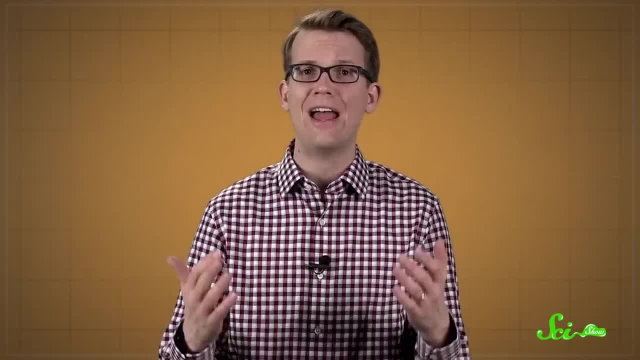 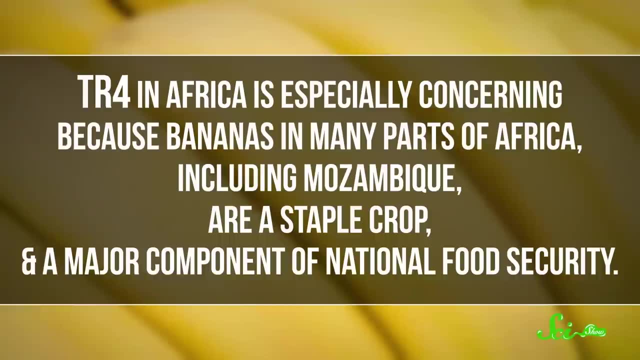 TR4 has reached the Middle East through Jordan and Lebanon, as well as Africa through Mozambique. TR4 in Africa is especially concerning because bananas in many parts of Africa, including Mozambique, are not just a tasty treat, they're a staple crop and a major component of national 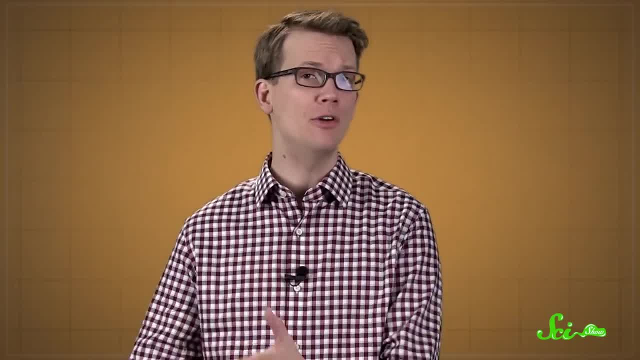 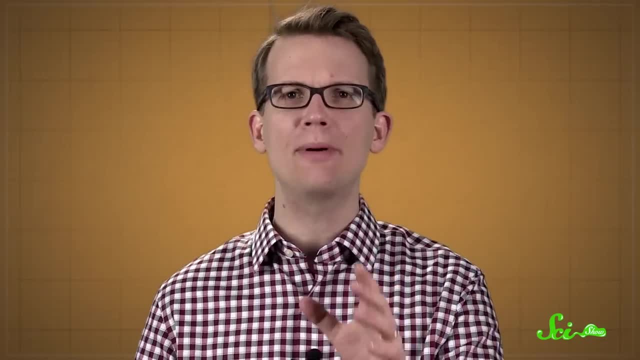 food security. Even worse, it seems likely that TR4 could also infect other varieties of African banana, many of which are grown as subsistence crops by rural families. What makes TR4 so dangerous? It's caused by a fungus that spreads through soil. If